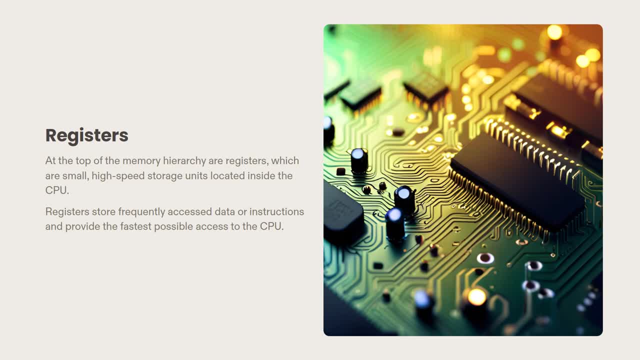 accessed data or the instructions and provide the fastest possible access to the CPU. The number of registers in a CPU varies depending upon its size and architecture, but they all serve similar functions, such as storing operands for arithmetic operations, keeping track of program counters and holding on to flags indicating certain conditions like overflow or carry out. 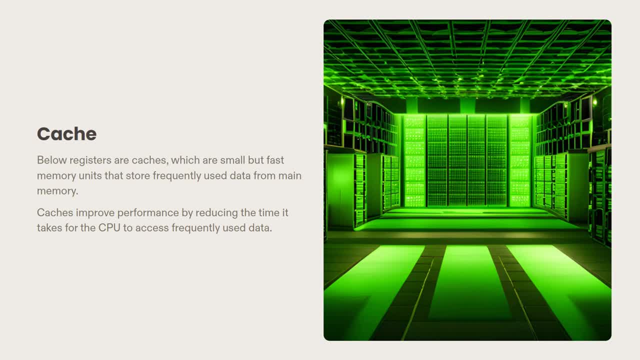 Now, below the registers, there are caches that act as small but incredibly fast memory units. They store frequently used data from the main memory and improve the performance by reducing the time it takes for the CPU to access frequently used data. This happens because accessing the data 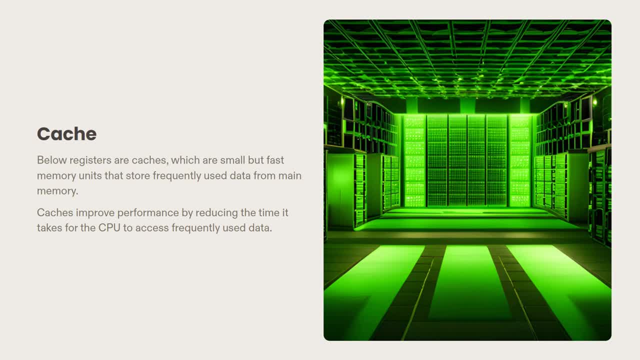 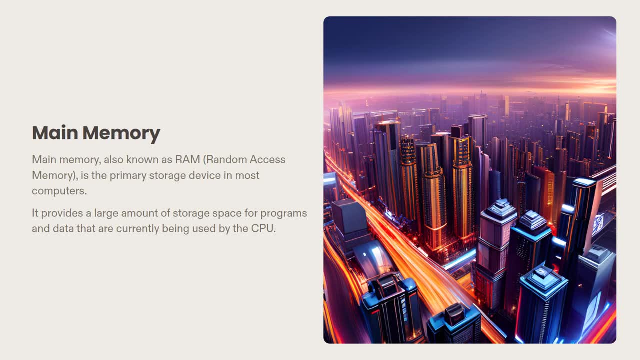 from cache is much faster than fetching it directly from the main memory. On the next level of the memory hierarchy, we have the main memory, which is also known as random access memory. It is the primary storage device in most computers and it provides a large amount of storage space. 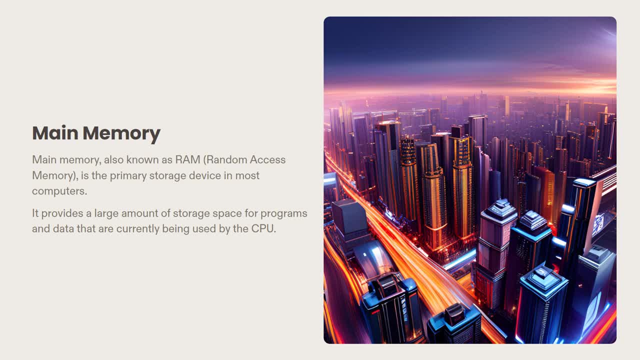 for programs and data that are currently being used by the CPU. Compared to secondary storage, main memory offers significantly faster read and write operations, making it ideal for storing data that needs to be quickly accessed and manipulated. It serves as the immediate working space for the 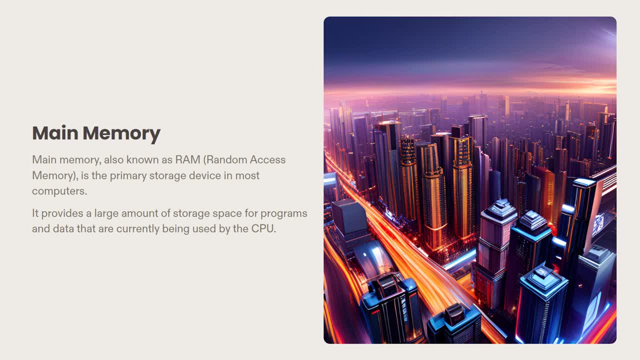 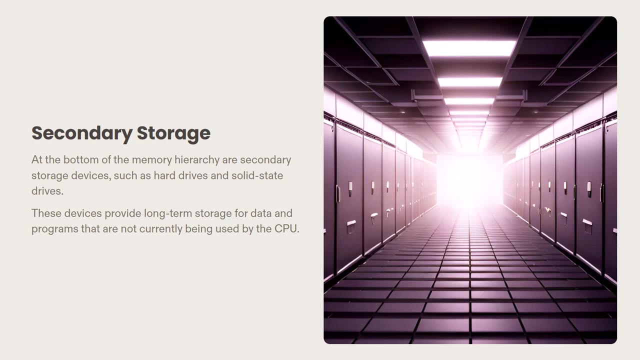 processor, holding both instructions and data that the CPU requires to perform tasks. In the last level of the memory hierarchy we have the secondary storage. Now these devices provide long term storage for data and programs that are not currently being used by the CPU. They are at the bottom of the memory hierarchy and are secondary storage. 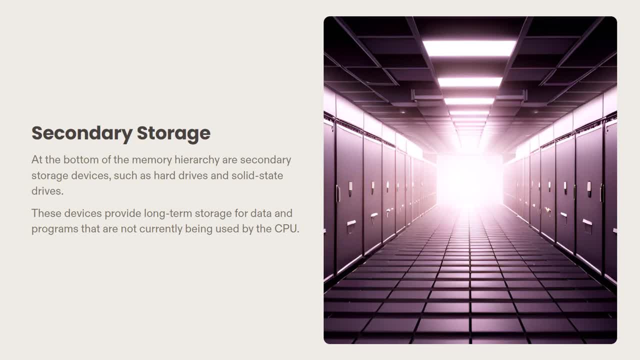 devices such as hard drives and solid state drives. Unlike main memory, secondary storage are non-volatile means they retain data even when the power is turned off. These storage devices offer a much larger capacity compared to main memory, but they are slower in terms of access speeds. The memory hierarchy with a